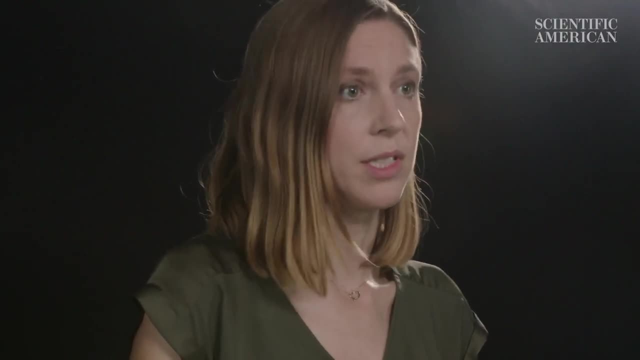 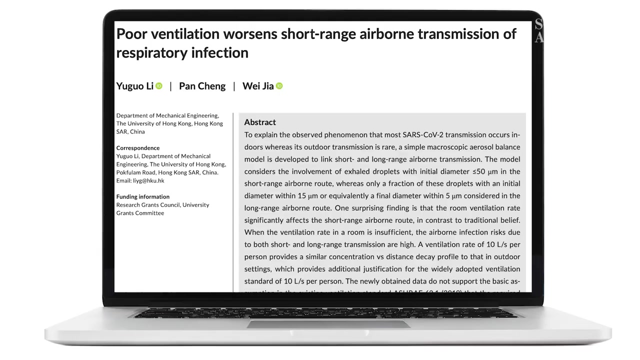 quality. ASHRAE standards aim to limit exposure to harmful substances with known exposure limits, such as formaldehyde, but not to pathogens. And here's the problem. According to experts, those air quality standards are far below what is needed to stop the spread of COVID. That's because 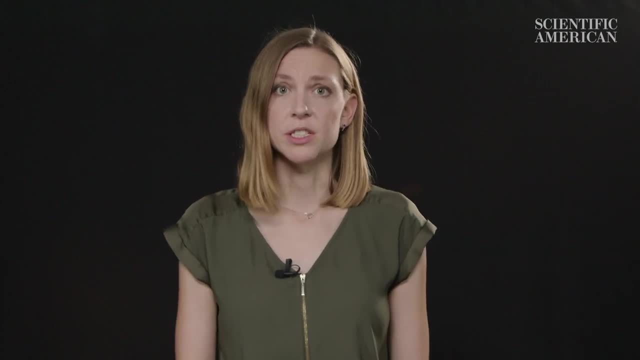 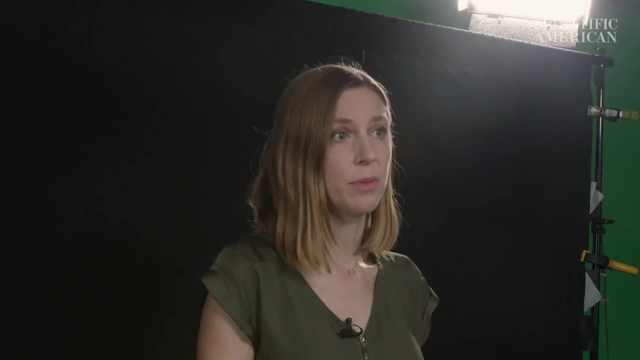 minimum ventilation rates don't totally stop the spread of airborne pathogens, and many buildings don't even meet those standards. Changing these standards takes time, but we're going to break down the components of improving indoor air quality and exactly what you need to do. 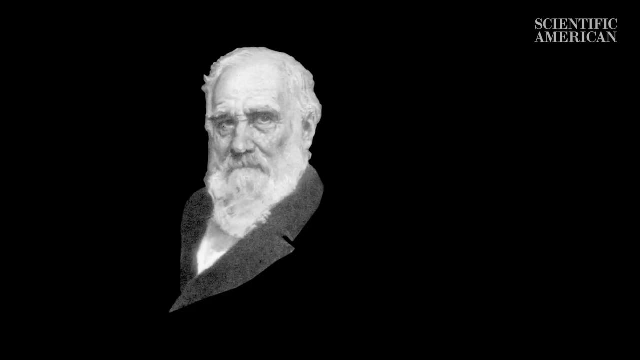 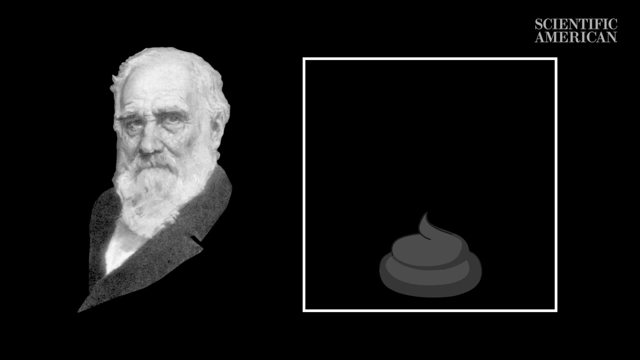 Number 1. Source Control. In 1858, chemist Max von Pettenkörper, one of the pioneers of the indoor air quality movement, said that if space contains a pile of manure, one should not try to remove the odor by ventilation. 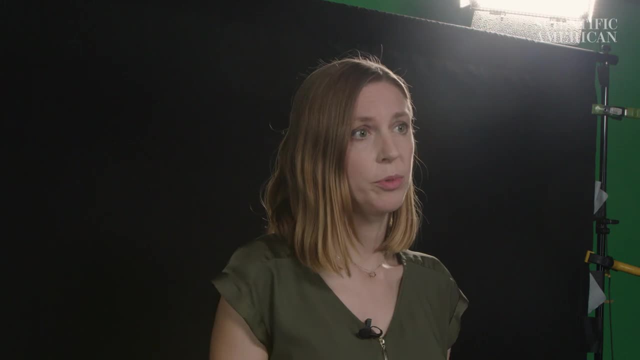 but rather remove the manure. For example, one could remove cooking gas fumes by using an electric stove instead of a gas one. So if you want to limit the amount of air you're using, you can use a gas stove instead of a gas one. So if you want to limit the amount of air you're using, you can use a gas stove instead of a gas one. So if you want to limit the amount of air you're using, you can use a gas stove instead of a gas one. So if you want to limit the amount of SARS-CoV-2, 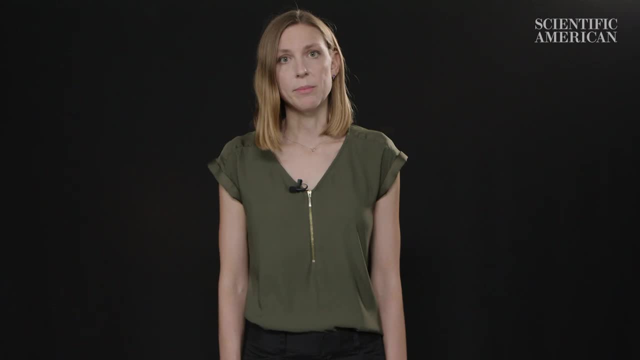 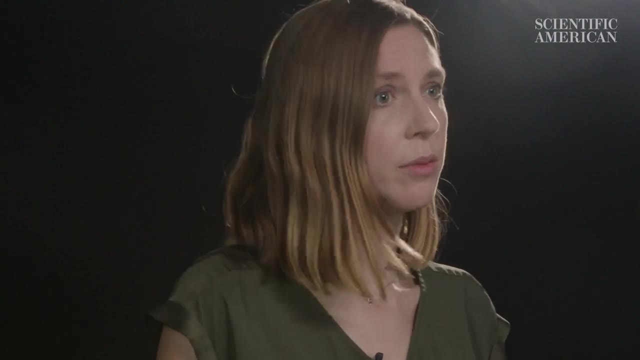 particles in the air. you could theoretically mandate that people wear high-quality masks and ensure that anyone who feels sick stays home instead of coming into the office. Of course, such measures alone cannot prevent all pathogens or other pollutants from entering the air, which is why other steps are needed. Number 2. Ventilation. 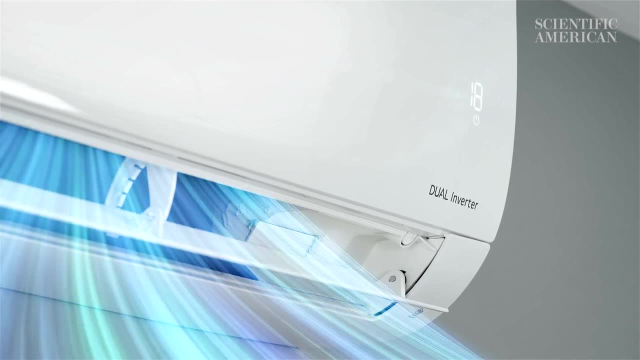 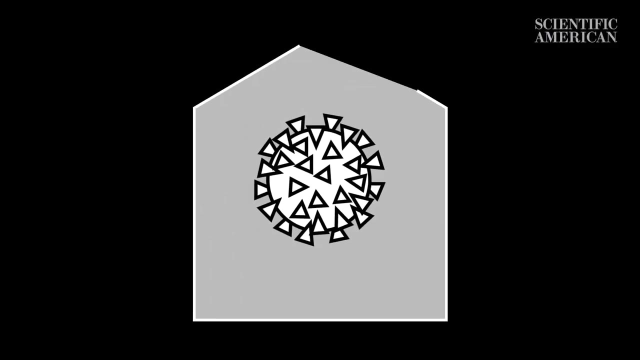 A building's ventilation level refers to how much fresh outdoor air is being brought in. This fresh air dilutes the concentration of virus-laden particles in the air. Imagine a SARS-CoV-2 particle indoors as a drop of food coloring in a cup of water. Outdoors it's more like a drop of 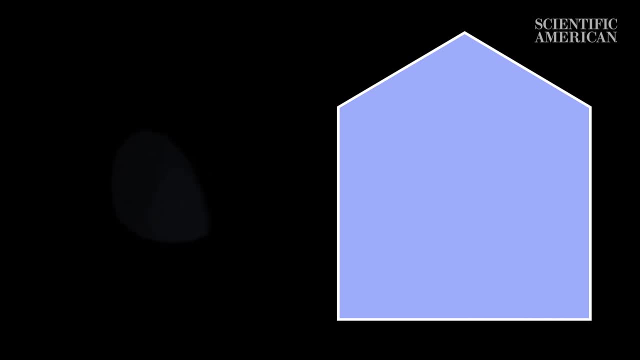 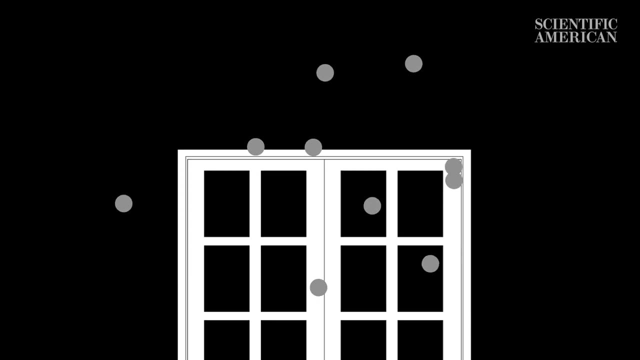 dye in the ocean. It rapidly becomes so diluted that it's largely undetectable. Ventilation makes the indoor cup a lot more like the outdoor ocean. The simplest and cheapest option is to open a window, but that's not always viable, especially if the air outside is more polluted than that. 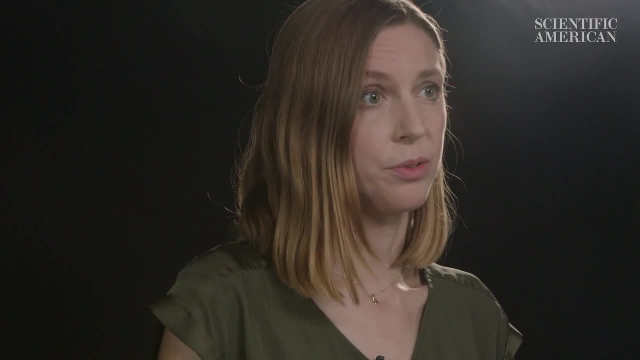 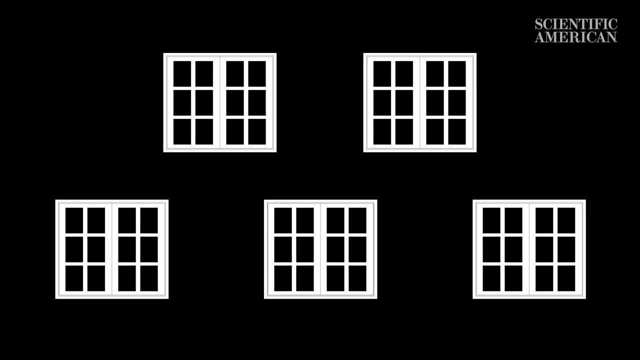 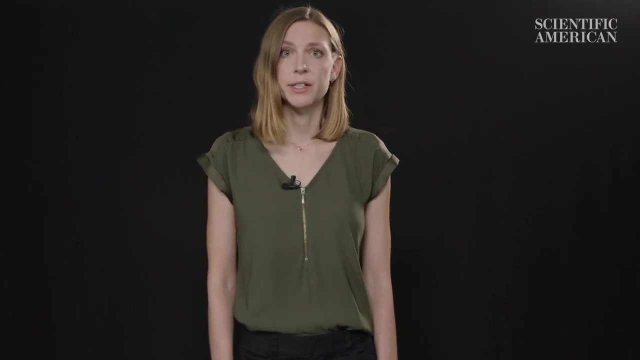 inside. Experts say this can become a major equity issue. People of color, for example, are more likely to live and work in areas where they're exposed to harmful pollution. Aside from windows, another source of indoor ventilation is an HVAC system. Most of these systems allow a building manager to vary the amount of fresh air intake. 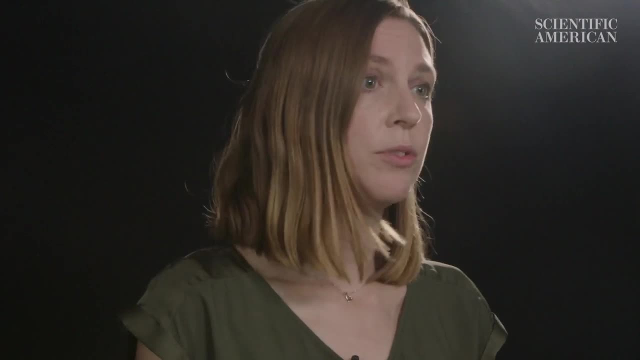 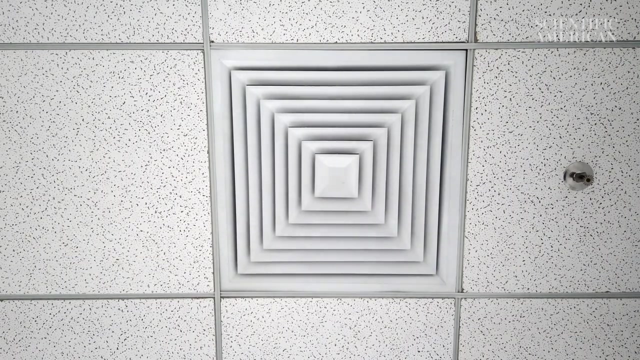 It should generally be set to maximum, experts say, provided the outdoor air quality is safe. Yet before the pandemic, many buildings had their HVAC systems set to recirculate old, stale air. A good rule of thumb is to aim for having at least six air exchanges per hour through ventilation. 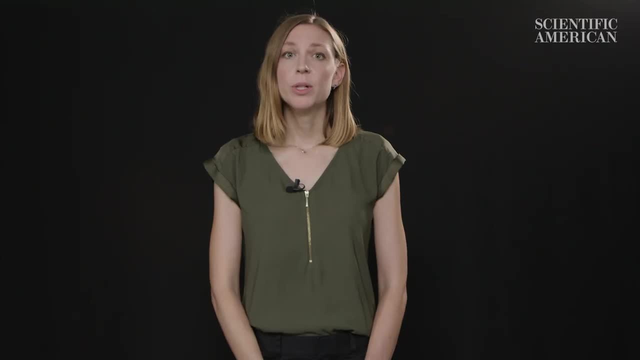 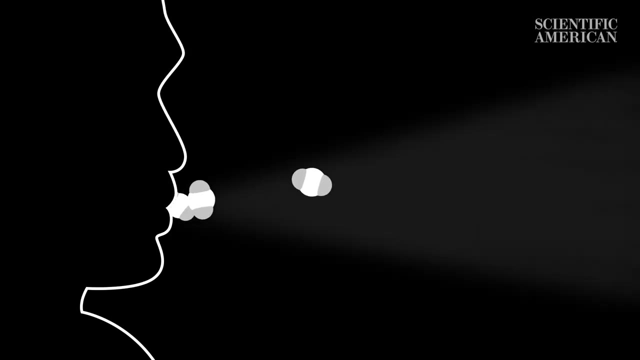 or the equivalent amount of fresh air through filtration. One way we can indirectly measure the amount of ventilation in the space is by using a carbon dioxide monitor. Humans exhale carbon dioxide when we breathe, so levels of this gas provide a good proxy for how diluted the air. 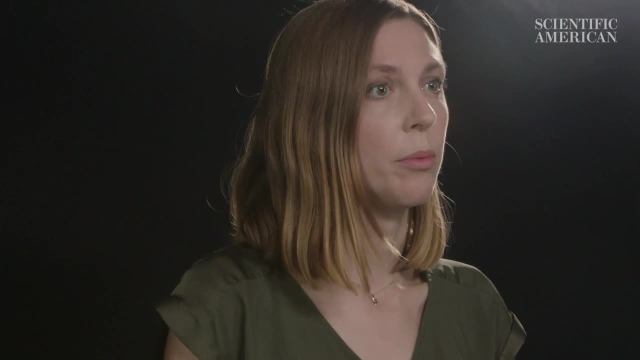 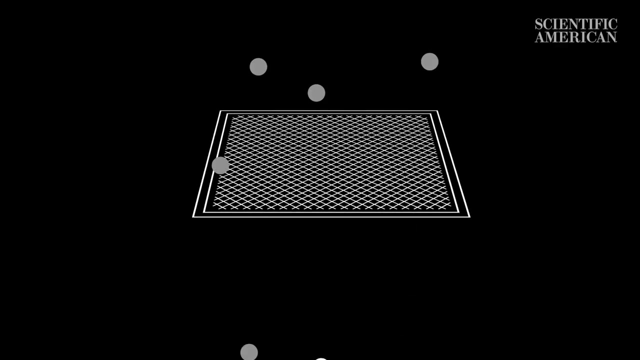 is, Values below about 800 parts per million are potentially well-ventilated. Number 3, filtration. Filtration basically just means removing particles and other pollutants from the air. A standard called MERV offers a way of comparing different filters. 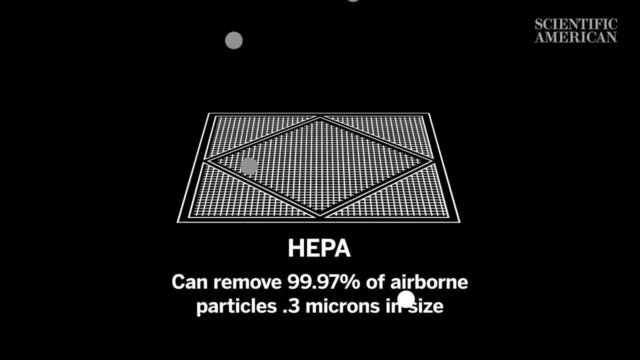 The gold standard filter, HEPA can remove 99.97 percent of airborne particles 0.3 micron in size and an even greater percentage of larger or smaller particles. HEPA is equivalent to a rating of MERV 17 or higher. A best practice is to upgrade filters. 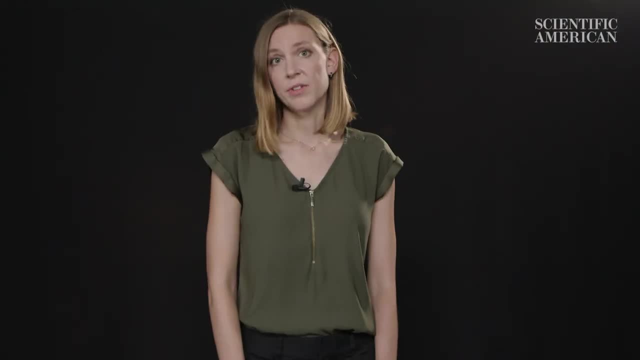 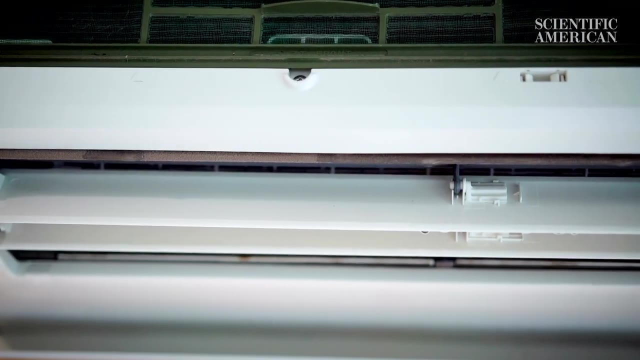 to at least MERV 13 for most indoor settings. Many HVAC systems can be upgraded to this standard, but some older ones may have trouble with high-efficiency filters and may cause air to leak around the filters. You can also buy a freestanding device called a portable air cleaner. 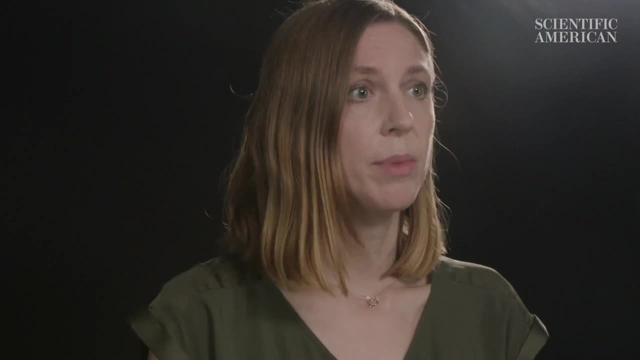 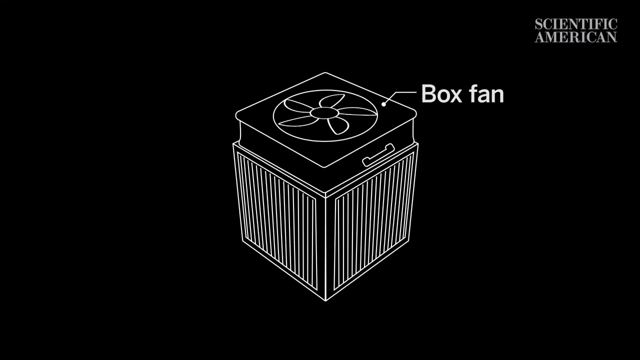 but these devices aren't cheap. Fortunately, researchers have come up with a more affordable solution called a Corsi-Rosenthal box. Basically, it's a DIY air cleaner made up of a box fan and four or five MERV filters duct taped together. You can even find the instructions online. It's 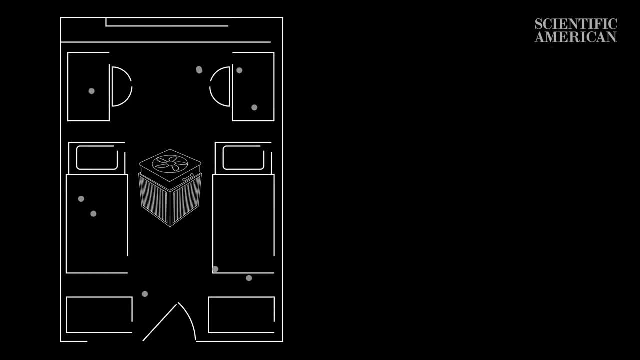 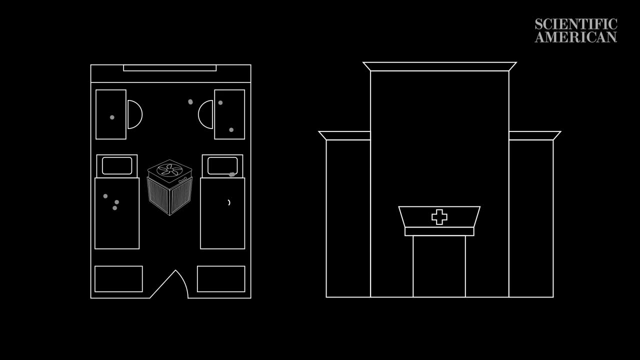 also pretty effective. A Corsi-Rosenthal box in a 200 square foot dorm room achieved the equivalent of about 24 air exchanges per hour, on par with a typical US hospital and better than many similarly sized portable air cleaners. Number 4, air disinfection. 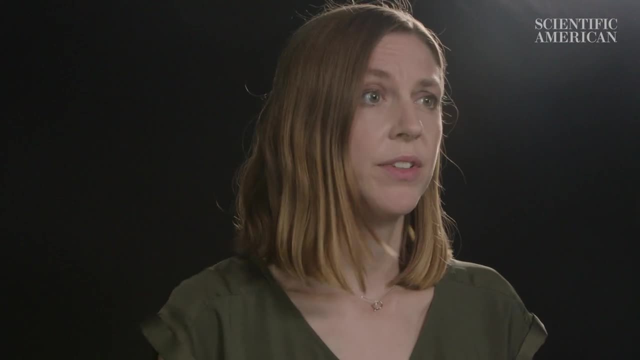 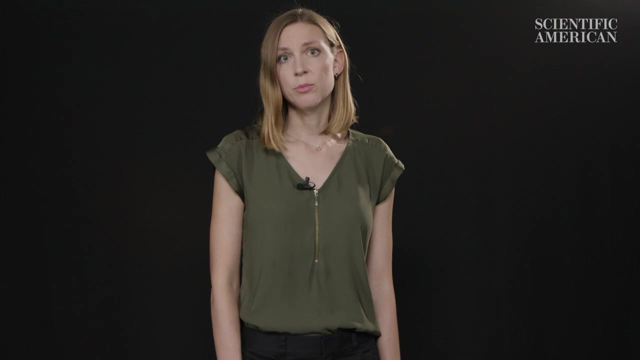 Finally, there's a method called air disinfection, which is basically inactivating viruses using ultraviolet light. Some systems work by shining a UV light across the top of a room, which neutralizes airborne pathogens as they circulate through that space.